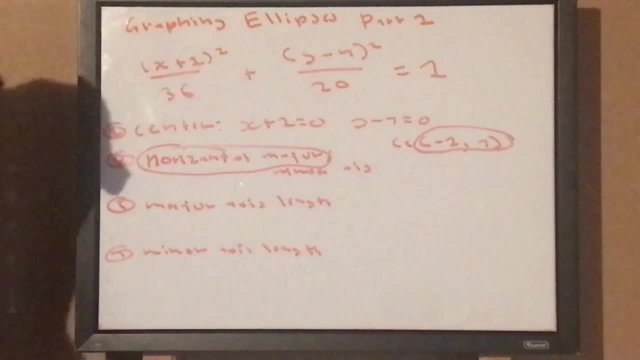 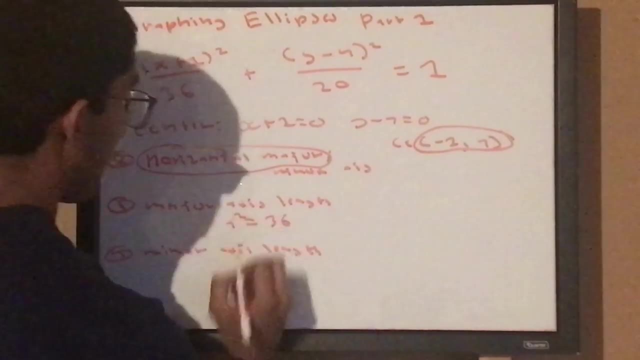 first that one, sorry, that one first. So how do we find it? We will set 36 equal to a, a square equal to 36, sorry. a is equal to six, And we will now multiply that by 36.. 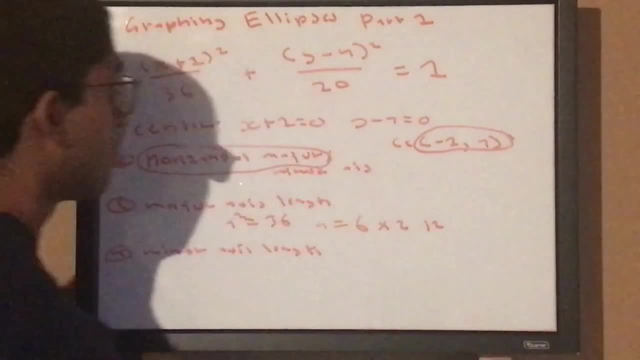 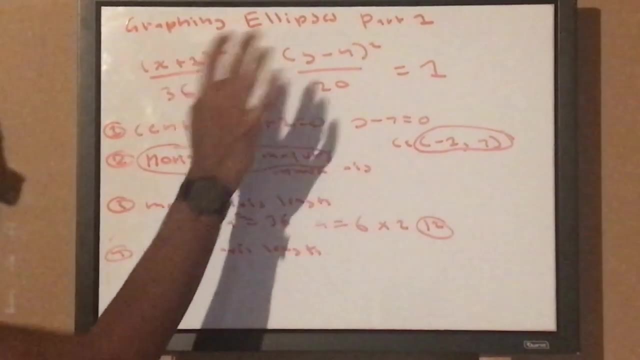 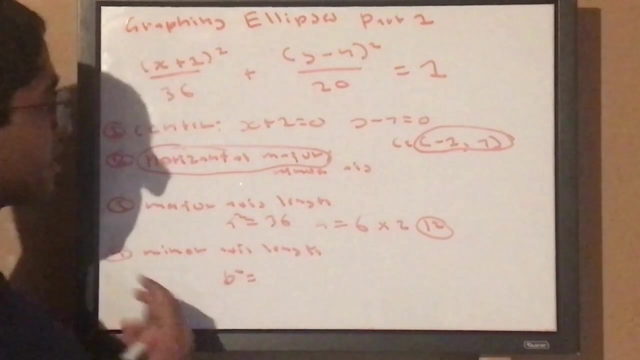 We will multiply six by two, which will give us 12.. So our major axis length is going to be 12.. And how do we find our minor axis length? So minor axis length is a fraction of the smaller denominator. Minor axis length is going to be, let's say b, square b, let b. 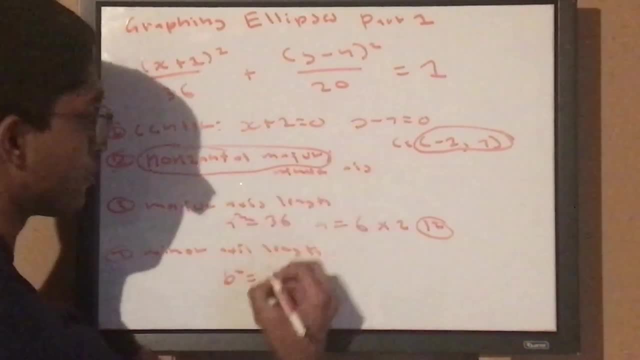 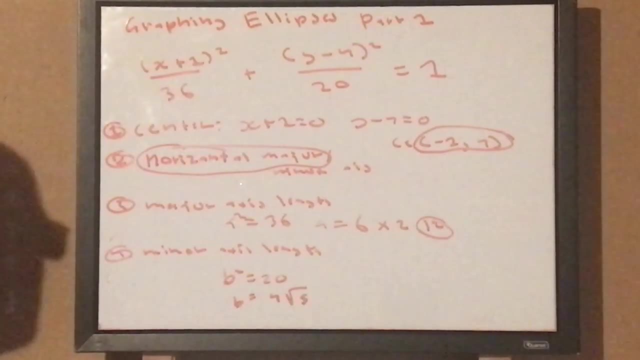 be our minor axis length. So b square is equal to 20.. b is equal to four root five, or sorry, two root five, And we will multiply this by two, And I'm not going to do that right now, but you can. 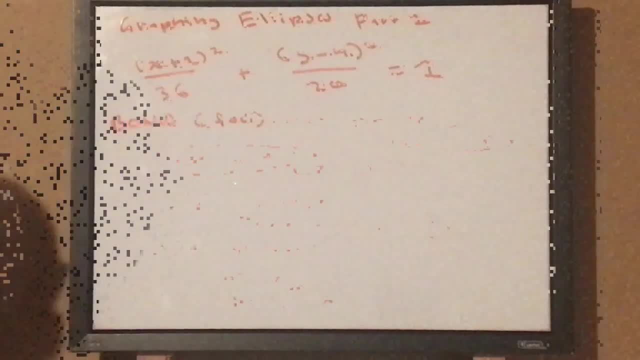 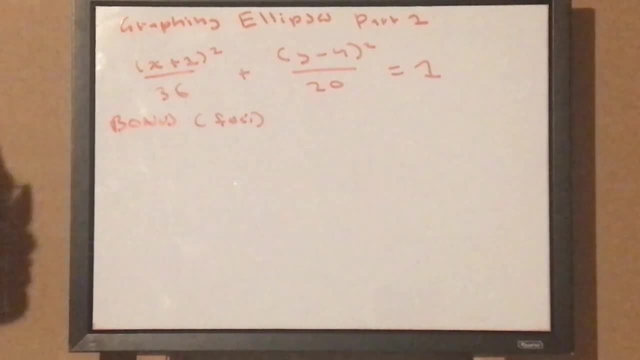 do that in your calculator and you will find your length All right. now that we've figured out our a and b points, we can figure out what's called foci. Foci are great reference points in your graph, on your ellipse. That's why I've included 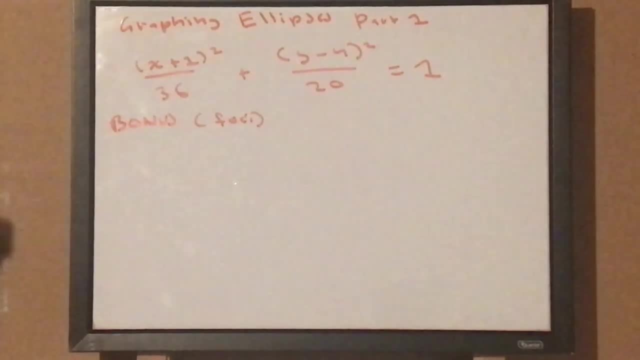 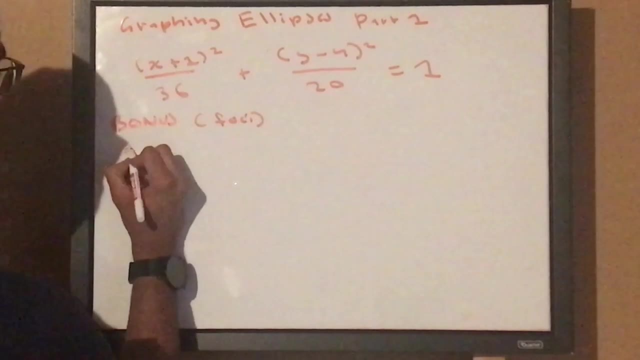 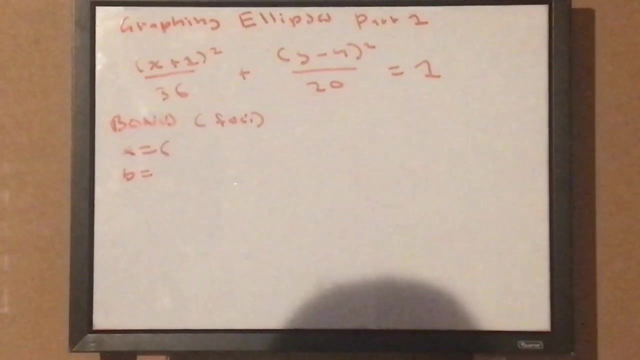 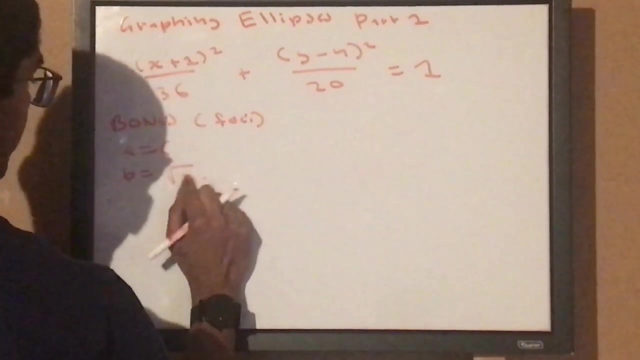 this bonus content for those who might want to use it, And it's highly, highly suggested that you use it because it makes it gives you a cleaner graph. So how do you find foci Recall: a was six and b was. b was root 20.. This was before we multiplied these values. 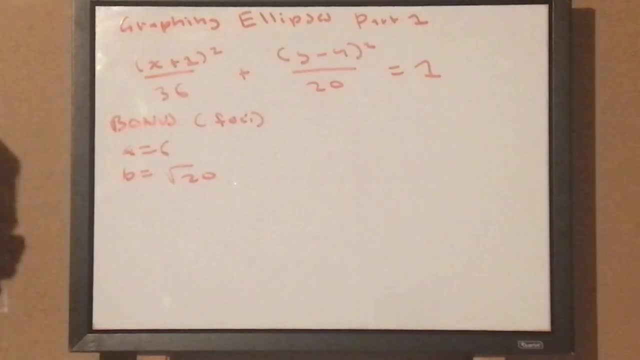 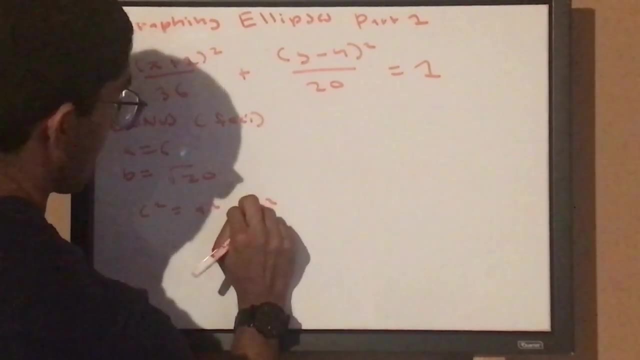 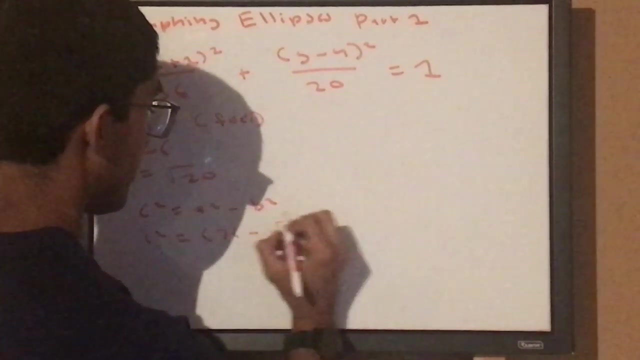 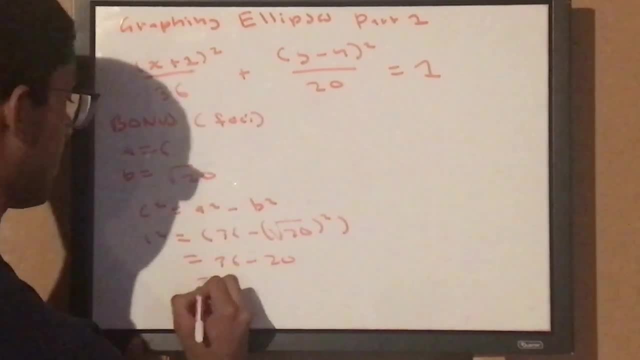 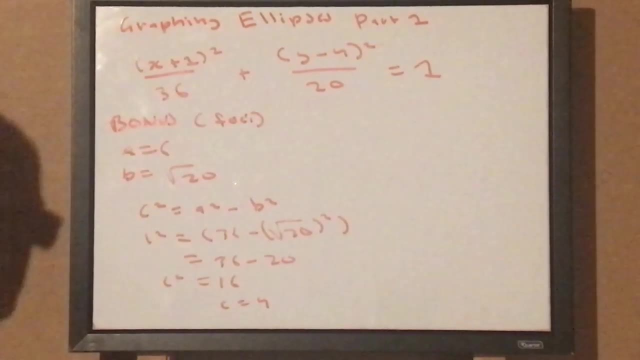 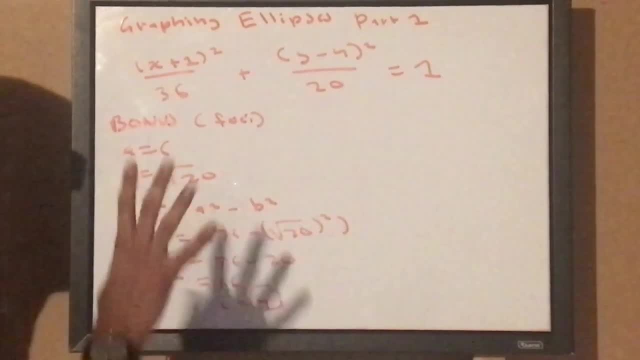 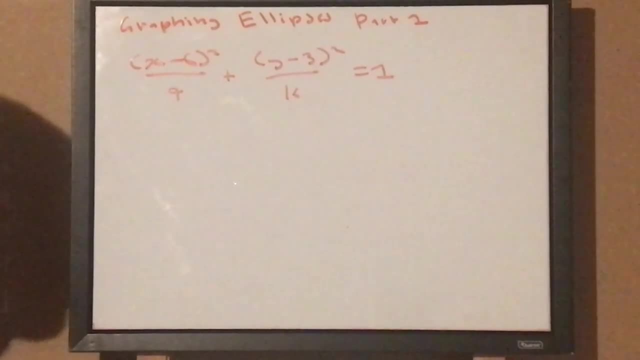 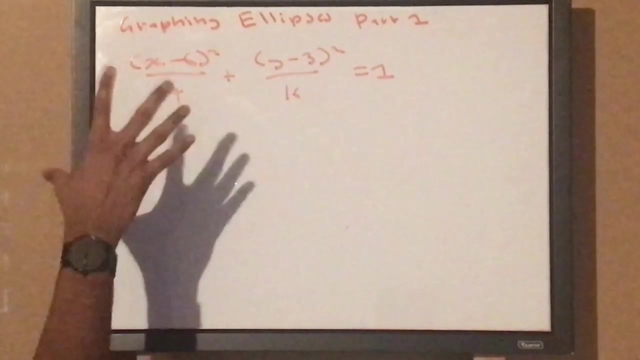 we found in this video. So make sure you come back to that. Alright, we've looked at example 1, we've figured out how to figure out the foci, the center, the major axis, lens. so let's go to our second example, which we'll repeat: the. 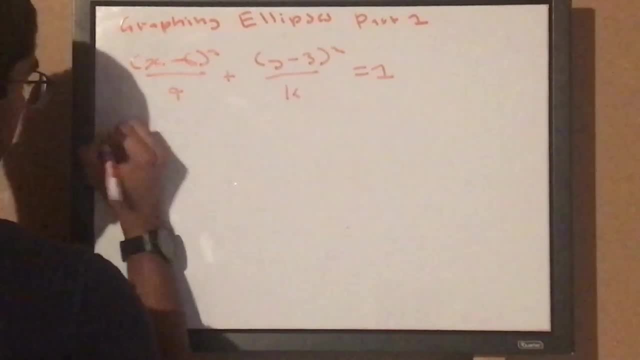 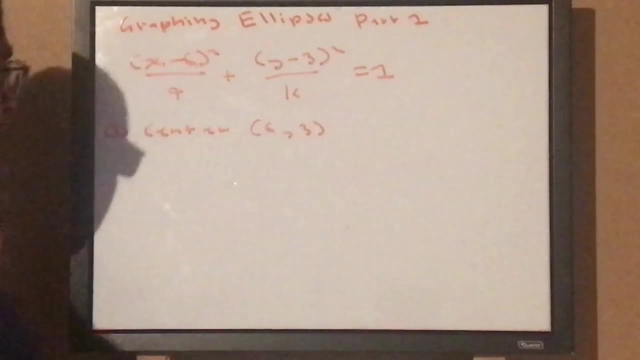 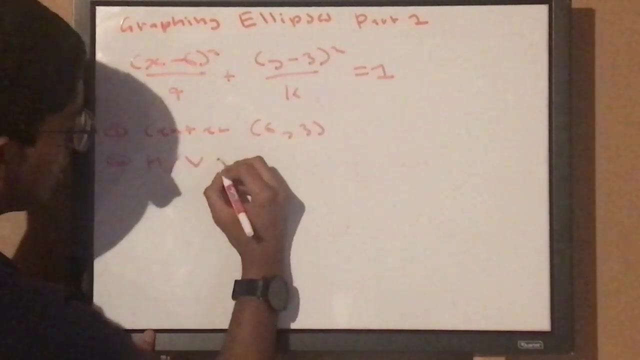 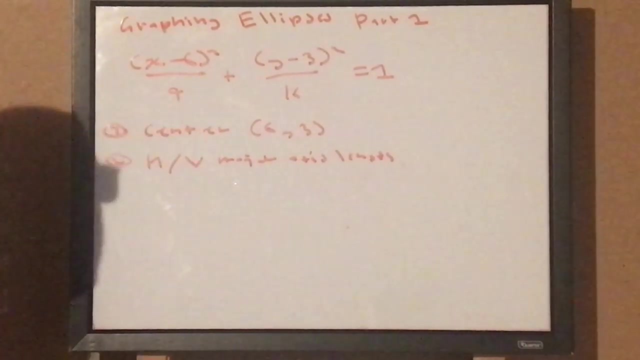 process so you get a more clear idea. So our first key component is our center, which is 6 and 3, remembering after we set those two to 0.. Our second key component is our horizontal slash vertical major axis lens. So in this case this fraction is the one with the bigger denominator and y squared. 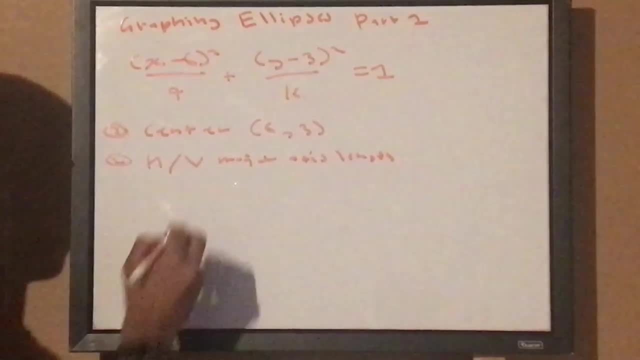 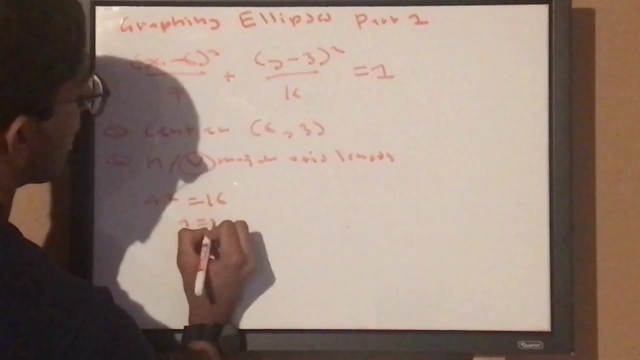 directly equates to a vertical major axis lens being found first. So we will do that. a squared is equal to 16,, a is equal to 4.. Multiply that by 4.. Multiply that by 2, and you get a is equal to 8.. 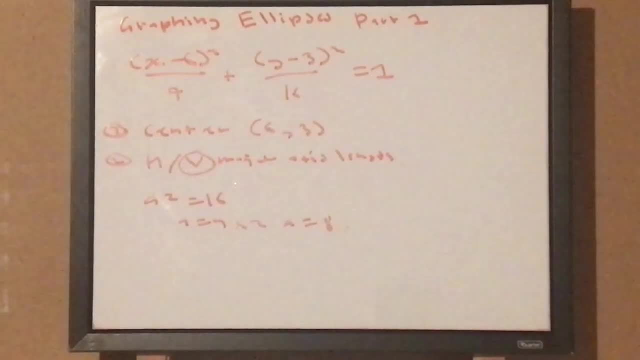 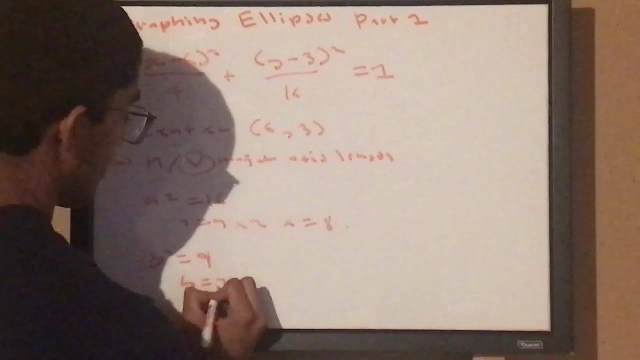 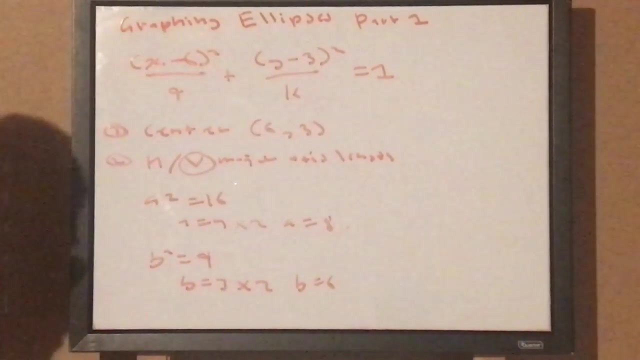 That is our first axis lens. so that's our major axis lens over here. b squared equal to 9.. b is 3.. Multiply that by 2, and you will get b is equal to 6.. That's our minor axis lens. 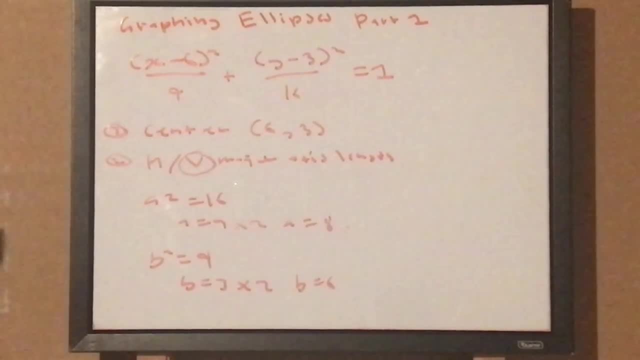 So now that we know a, which is our major axis lens, and b, our minor axis lens- 8 and 6 respectively- Let's graph our ellipse. but we also have to find our foci, So let's go over foci real quick. 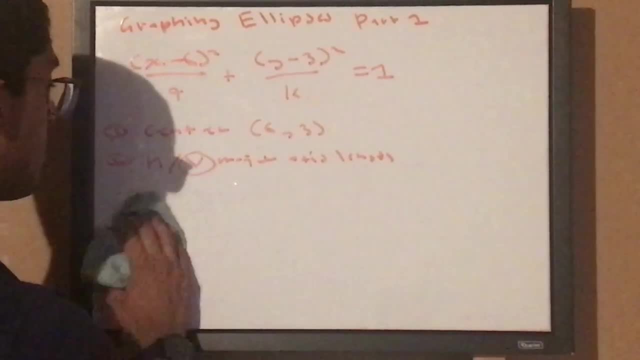 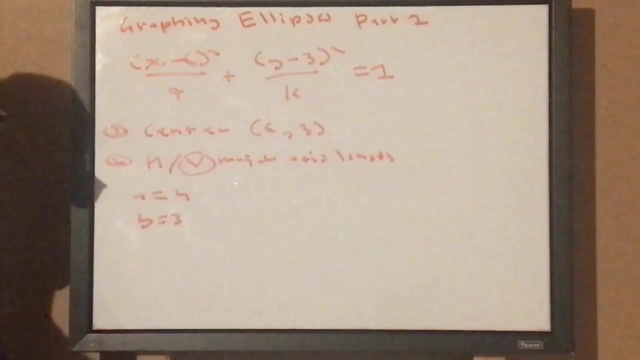 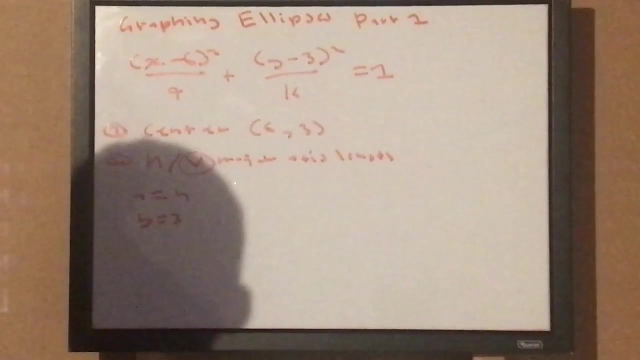 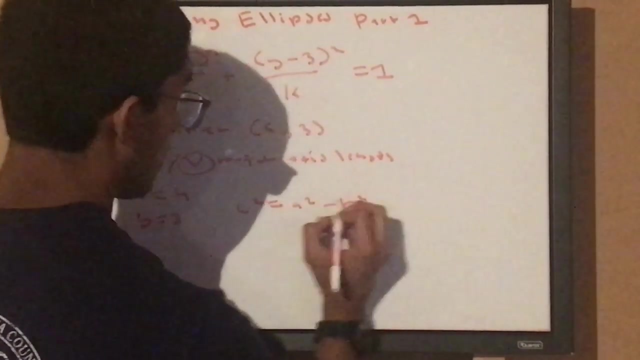 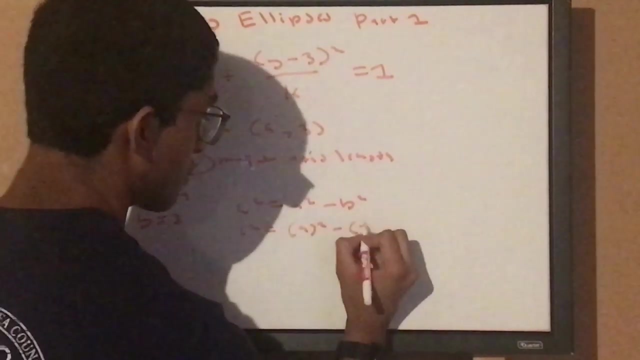 a was 4, b was 3, let me just make sure of that real quick. Yep, that's right. Okay. So let's bring back our foci. Let's bring back our old handy-dandy formula: c squared is equal to a squared minus b squared, 4 squared minus 3 squared. 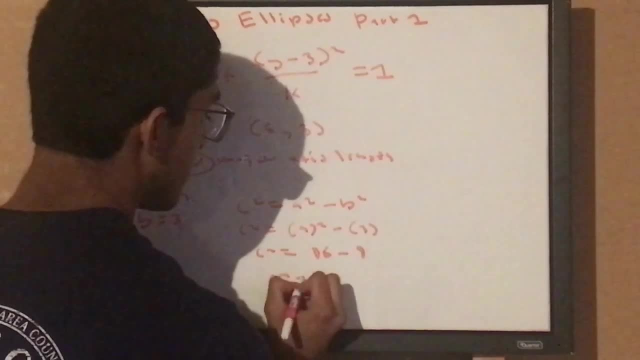 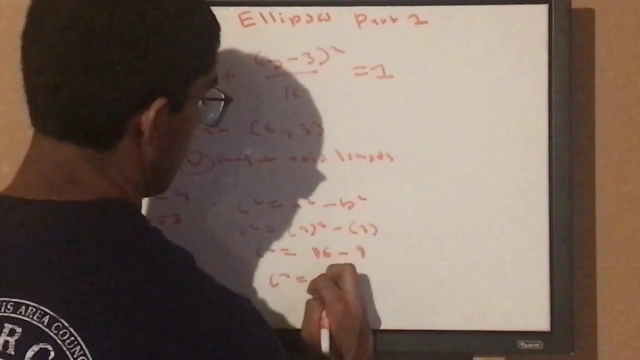 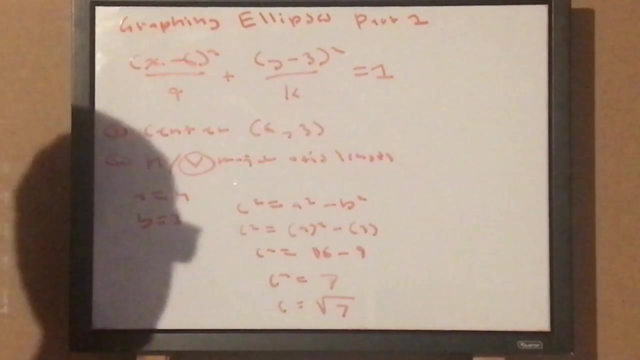 c squared is equal to 16 minus 9.. c squared is equal to 7.. c is equal to root 7.. root 7 is going to be 7.. root 7 is going to be 7.. We are going to be our foci. 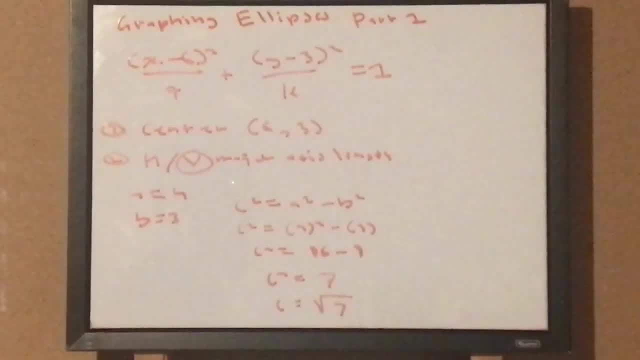 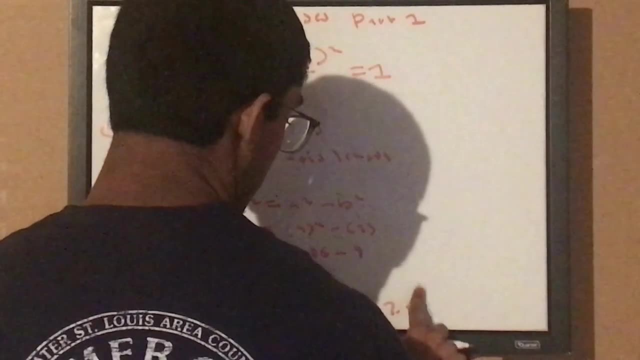 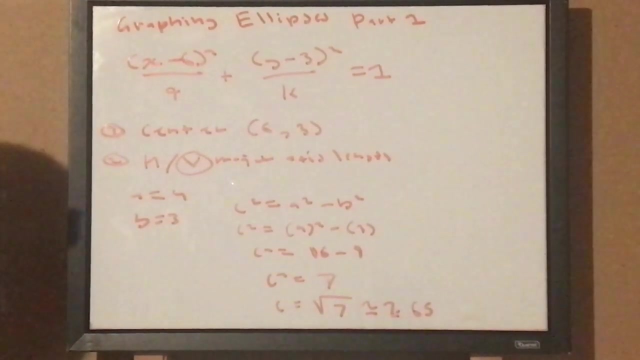 Let me just give you a decimal for that value, That is around 2.65.. There you have it, ladies and gentlemen. We found the foci, we found the a values, we found the b values, the lens which was: 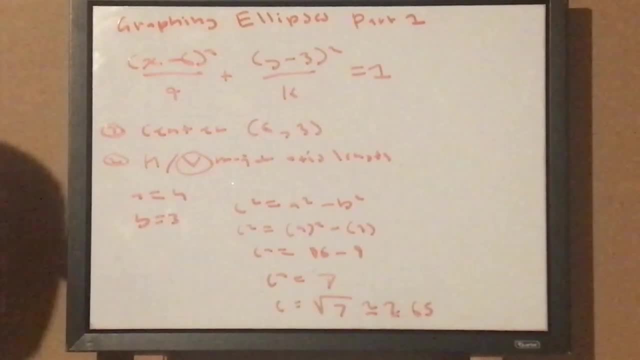 the previous cut. Yeah, Let's go on with the third example. All right, guys, Let's go on. go on to a third example over here. so you might be like: this looks a little familiar, right? it looks like the equation of a circle and you're. 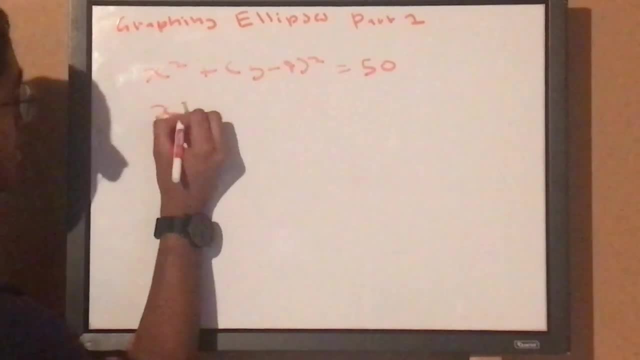 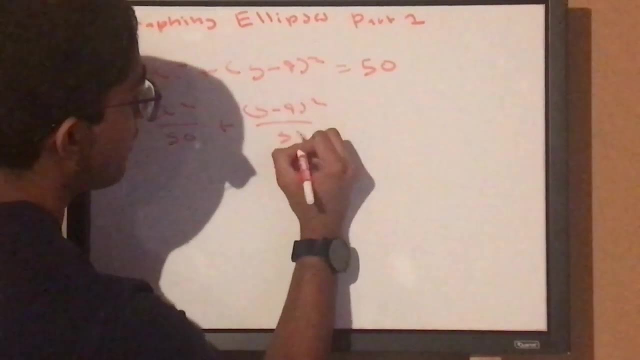 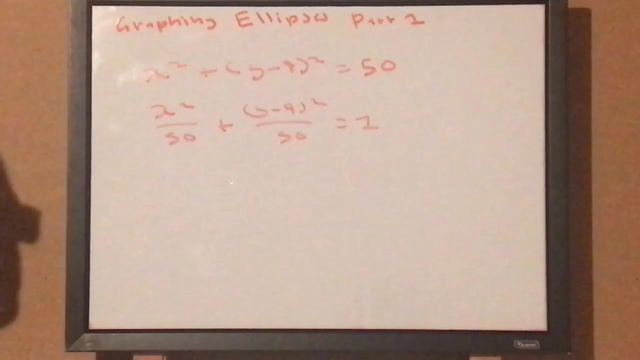 absolutely right. essentially, what we have here is x square over 50 plus y minus 9 square, or 50 equals to 1. this is just another way we can write that, and in this ellipse standard form, we see that a is equal to b. therefore, this ellipse is actually a circle, so let's figure out how to find. 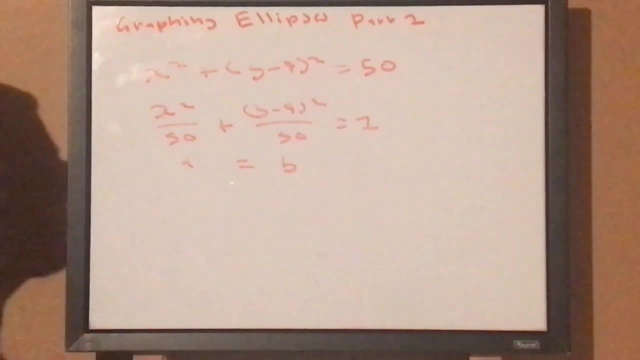 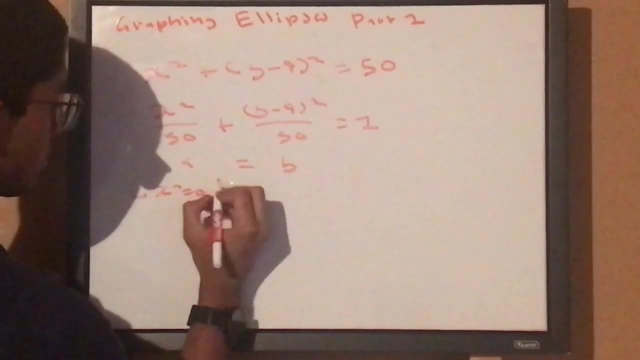 the key components in order to graph a circle. technically, this ellipse is a circle, so the first thing we have to find is the center. you can find the center by setting: x squared is equal to 0, x is equal to 0, y minus 9 equal to 0. 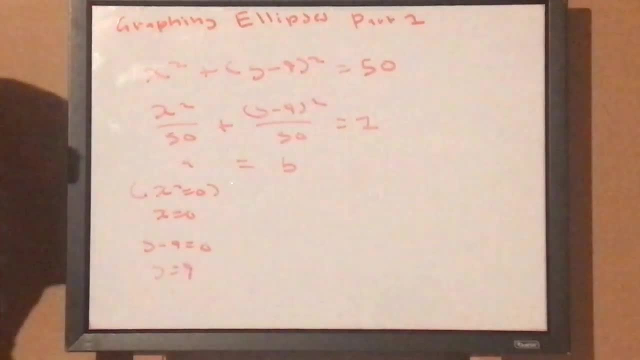 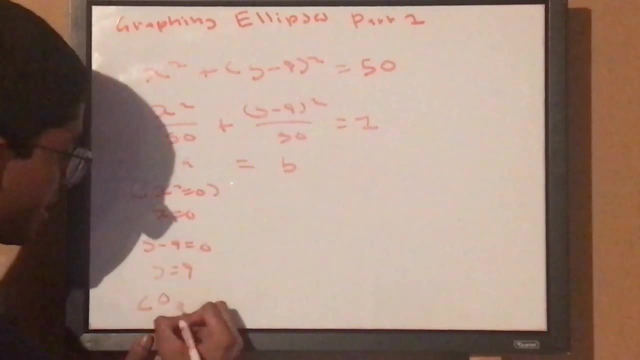 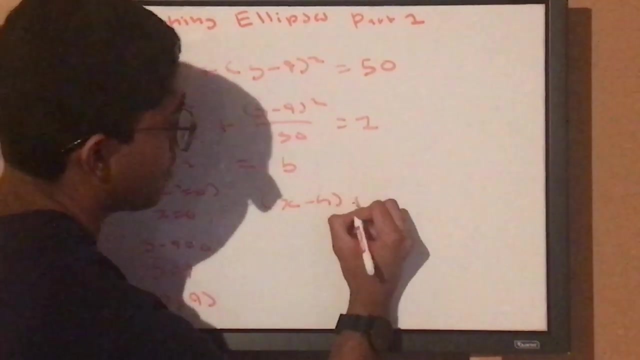 move 9 to the other side, we have: y is equal to 9. now that we have our x and y values, we can find the center slash, the vertex of the circle, which in this case is 0- 9. how do we find the radius? recall that the standard form for a circle is x minus h. 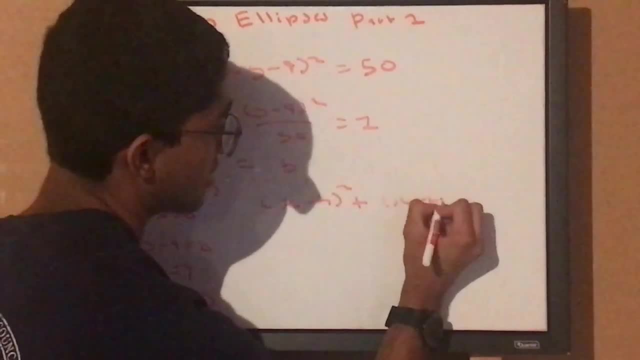 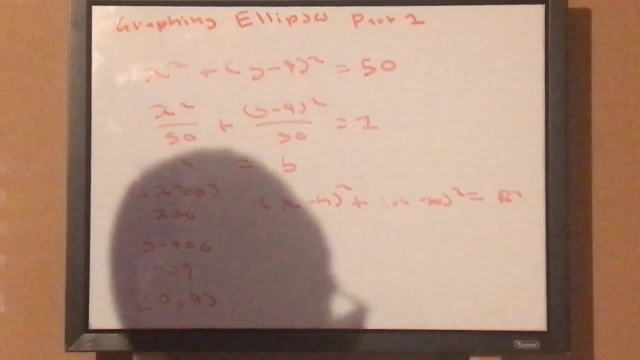 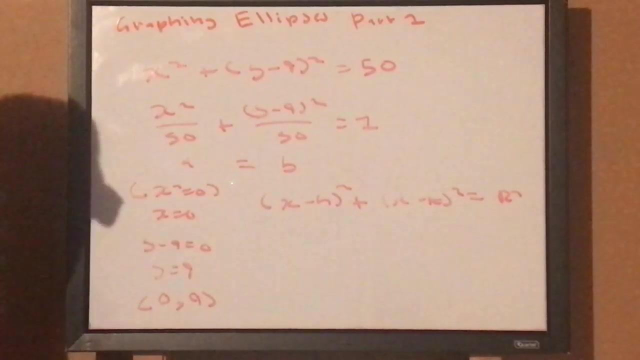 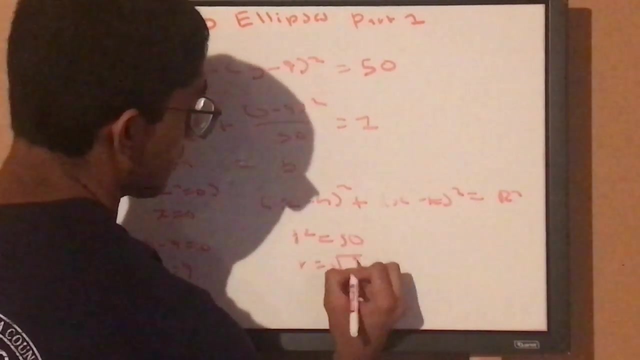 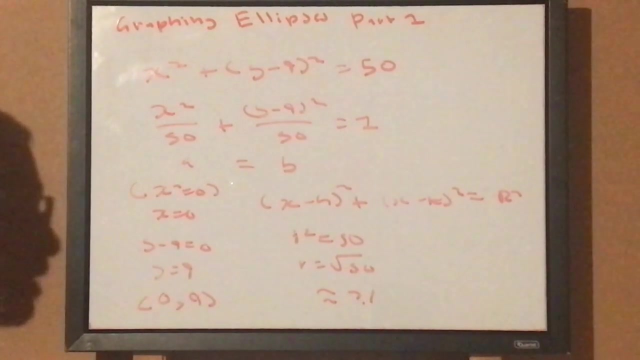 plus x minus h square plus x minus k square is equal to R square. yeah, that's it. so R square is equal to 50. R is equal to root 50. just about 7.1, boys. that's it. thanks for watching my video. make sure to subscribe and watch out for part 2 and I am out.